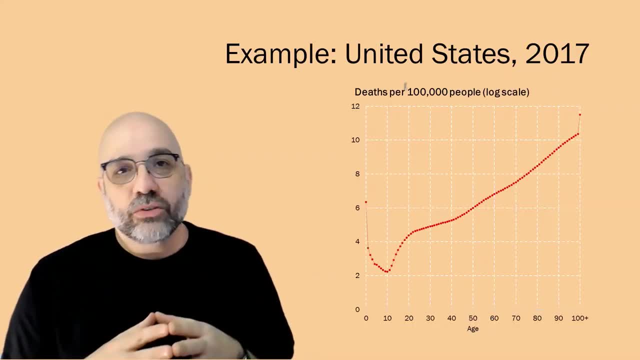 through one period in time. For our example, we'll start with the mortality rates for every age in the United States in 2017.. I've converted the death rates to a log scale here so we can see the fine differences at very low rates of mortality. 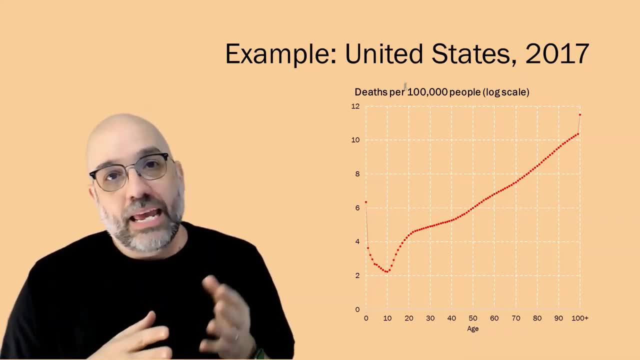 The fifth ratio is the fertility rate which we have at young ages. You can see that age are 0 is the most dangerous year in the early part of life, when a little more than one half of 1% of American babies died in their first year of life in the year 2017.. Those who made it out of that year 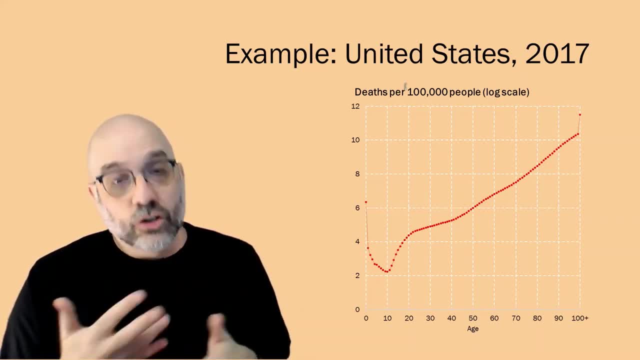 experienced much lower death rates through their early years, Until in their teen years, the death rates start rising. People experience accidents, violence and so on, And then later in life, of diseases- diseases of old age- start to come into play, like diabetes and hypertension. and 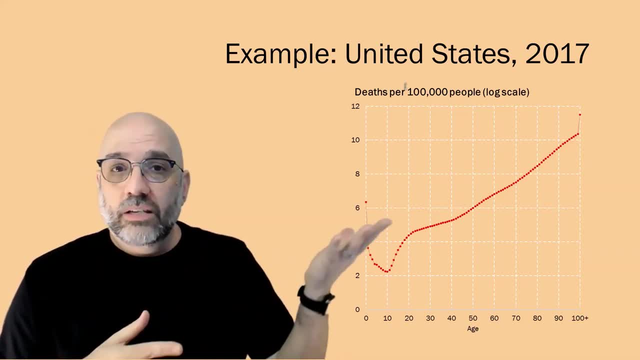 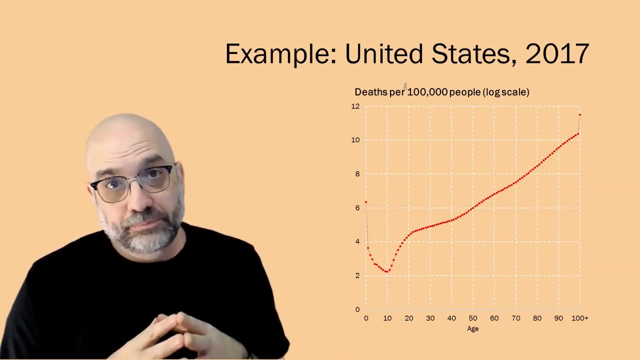 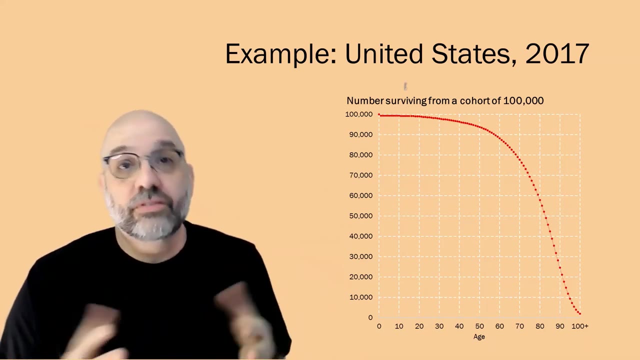 cancers and heart disease, until by the older ages, the death rate has risen and risen and risen until finally, at the very end, everybody will be dead. So we'll take our hypothetical cohort, 100,000 individuals, and we'll subject them to those observed mortality rates that we saw in the year 2017 in the United States, We lose about a half of 1% in that first year of life. then we don't lose very many more for the next 10 or 15 years and eventually you see them start to. 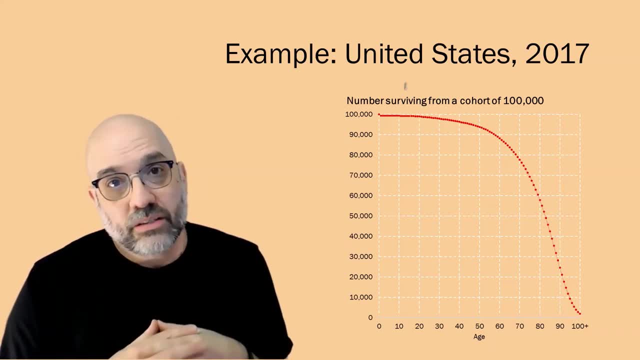 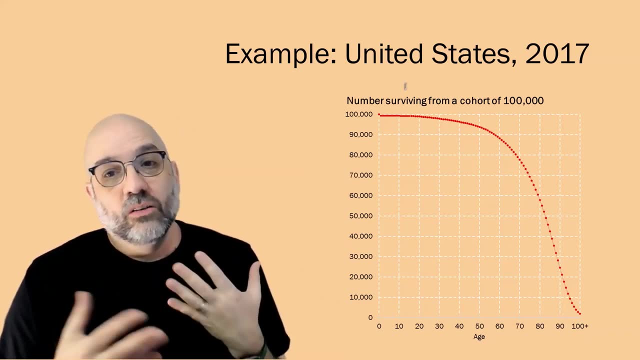 drop off as mortality rates eventually rise. You don't get below 90,000 of that 100,000 member cohort until almost age 60, and then you see the mortality rates as they rise. we start to lose more and more until you get. 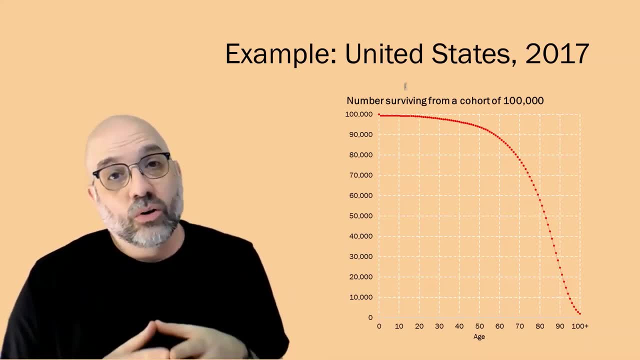 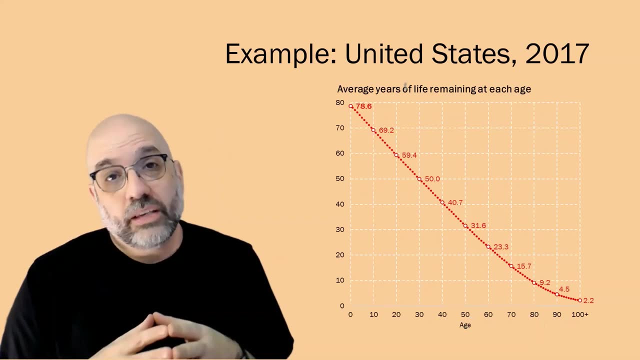 eventually all the way down to zero members of the cohort left after age 100.. So just looking at the experience of those 100,000 people, we can calculate how long the average member of that hypothetical cohort lived. In this case, United States 2017, the average member of that hypothetical 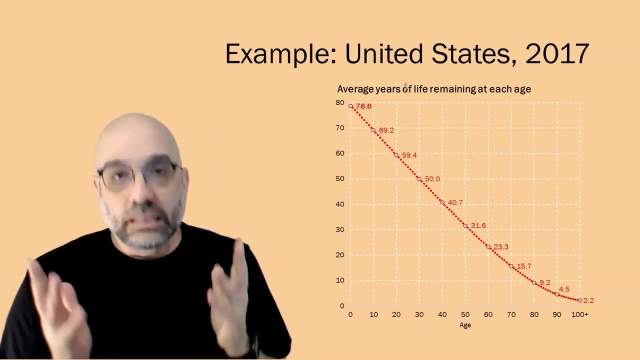 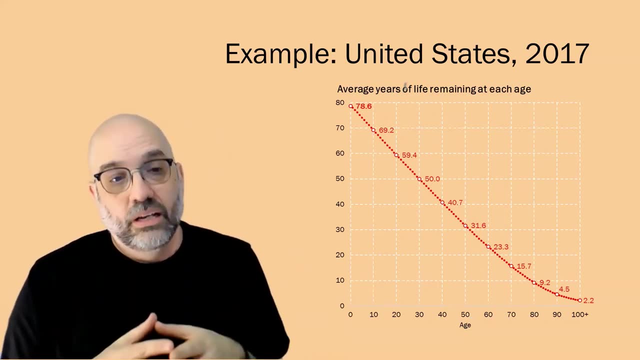 cohort lived 78.6 years. That was the life expectancy in the United States, that top line number that we hear so much: life expectancy 78.6.. Technically it's life expectancy at age zero, but we usually just call it life expectancy. 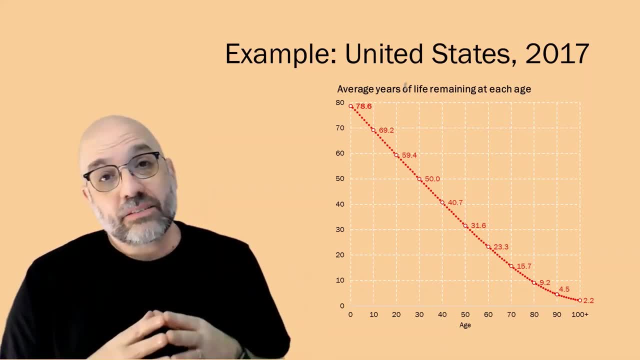 One thing you can see is that as soon as you make it past that first year of life, you can start to expect to live longer than the life expectancy at age zero. For example, people who live to age 20 in our figure have a life expectancy of 59.4 years left. That's the 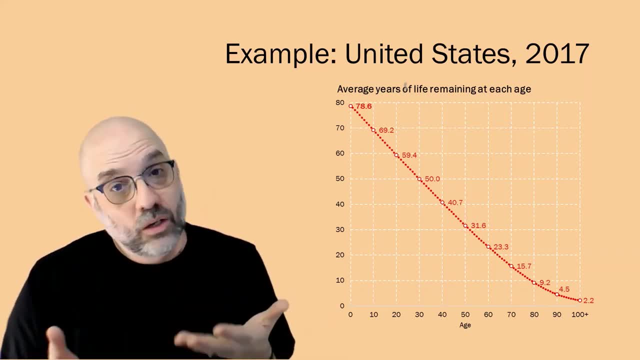 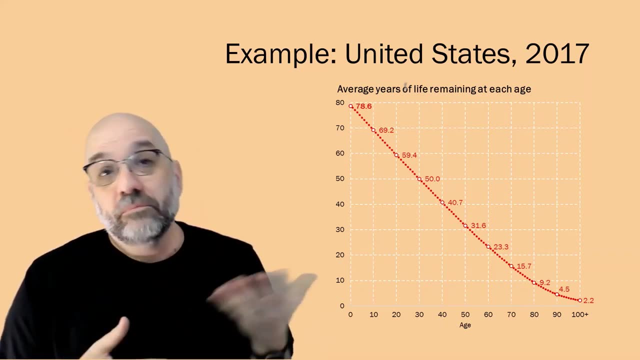 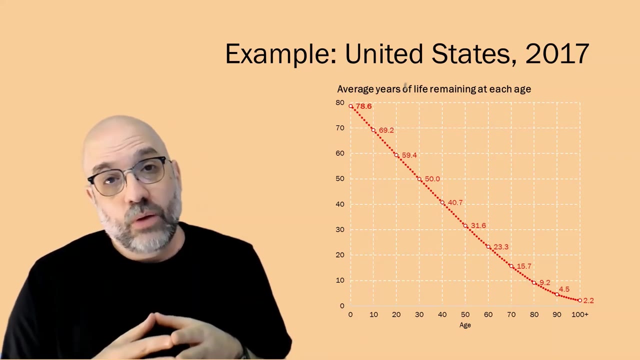 average years left for people who reach age 20, which will get them up to age 79.4 on average. If people live all the way up to age 70 in this hypothetical cohort, you see, on average they will have 15.7 years left to live, which will get them to age 85.7.. In fact, some people live past age. 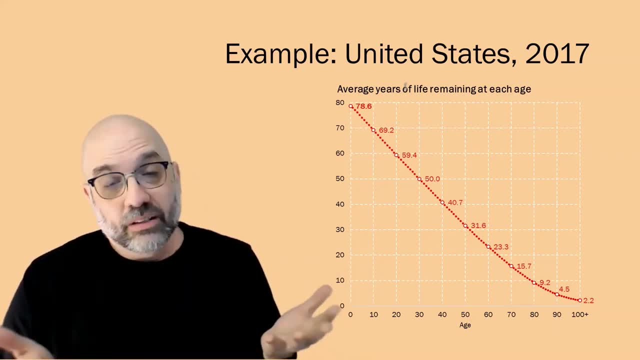 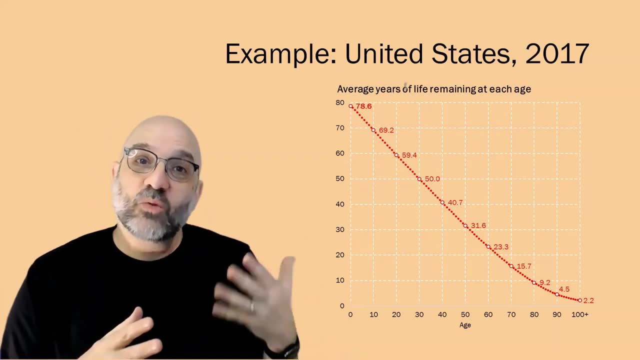 78.6 altogether, and those people obviously are expected to live beyond age 78.6.. Using our data from 2017,, if you make it to age 100 in the hypothetical cohort, you have an average of 2.2. 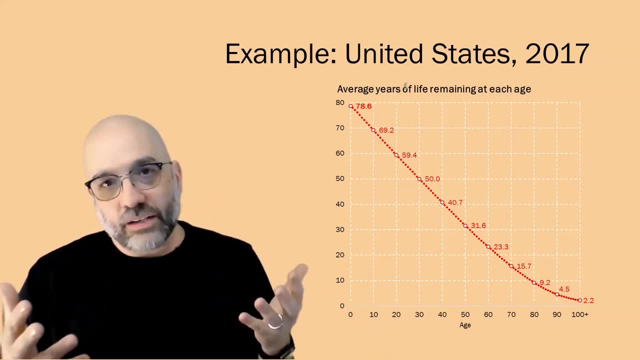 years left to live. This is why it's not correct to say I'm 75 years old. I live in a society where the life expectancy is 78.6,. therefore, I have 3.6 years left to live Once you've made it to age 75,. 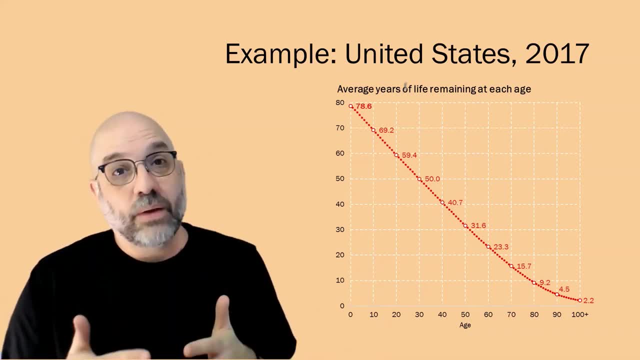 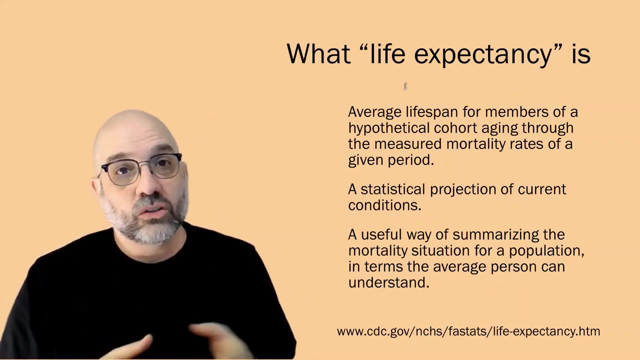 your life expectancy is considerably higher than the life expectancy at age zero. So we return to what life expectancy is the average lifespan for members of a hypothetical cohort aging through the measured mortality rates of a given period. That statistical projection of current conditions gives us a good picture of what the mortality experience of that population is, without giving